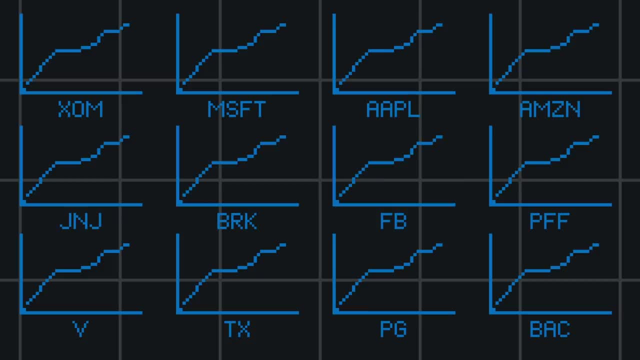 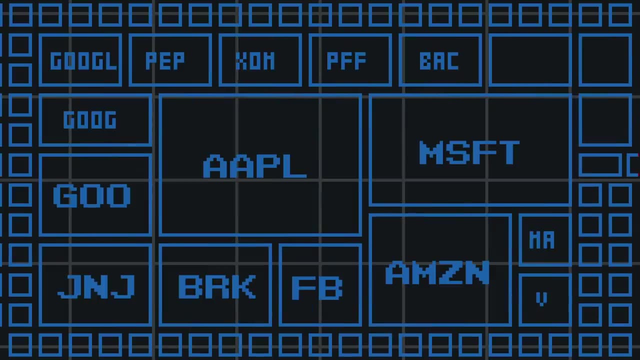 The S&P 500 is a measure of the average performance of 500 of the largest companies in the United States, weighted by company valuation, meaning that companies with a higher market value have a larger effect on the S&P. Again, market value corresponds. 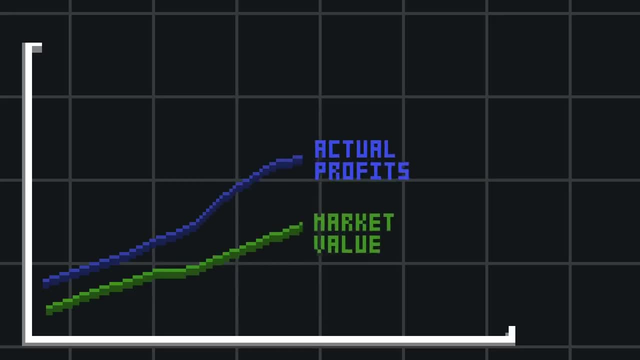 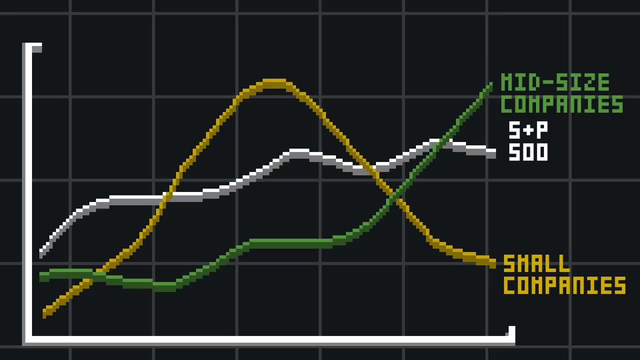 to what investors believe a company is worth, rather than actual profits. The S&P doesn't directly represent the market as a whole. Many small and mid-range stocks can fluctuate according to different patterns. Still, it's a pretty good proxy for the overall market. 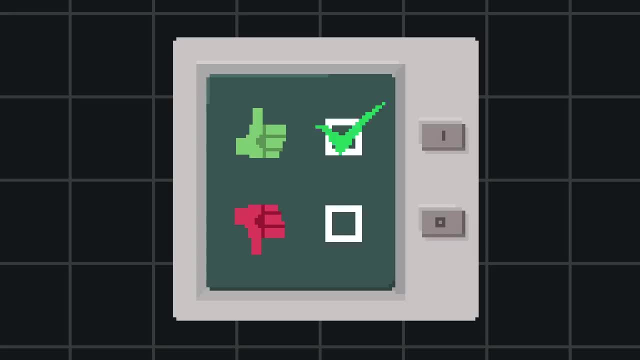 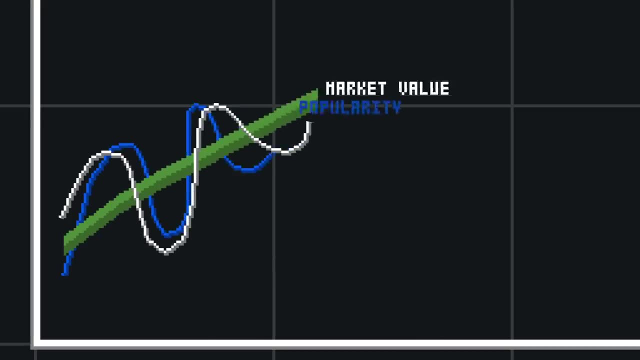 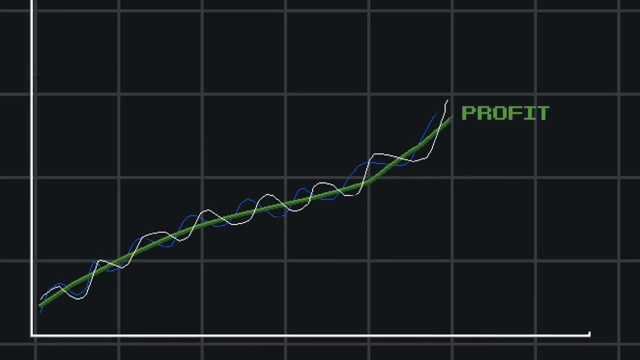 It's often said that the stock market behaves like a voting machine in the short term and a weighing machine in the long term, meaning, short-term fluctuations in stock prices reflect public opinion, But over the years, in the longer term, they do tend to actually reflect companies' profits. 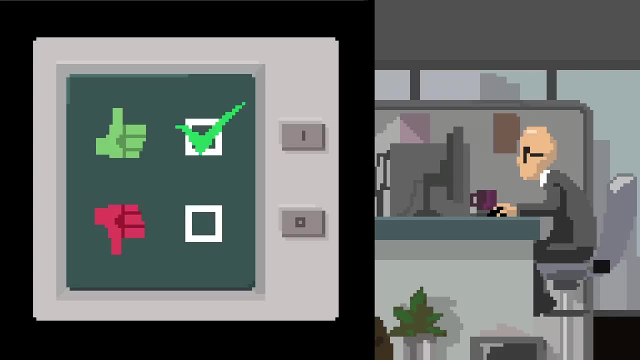 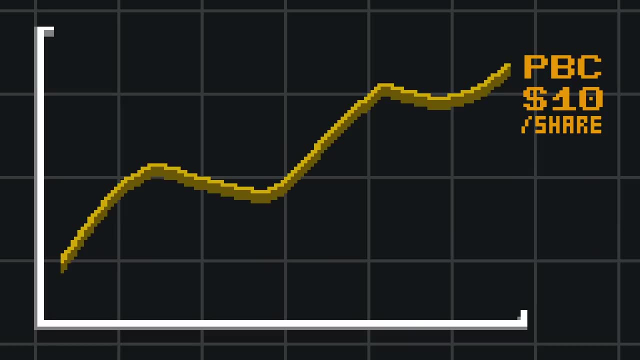 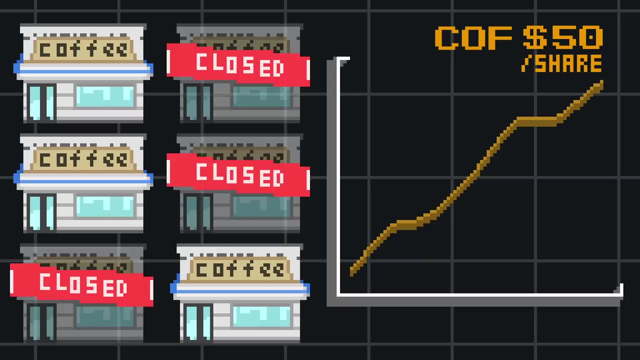 Active investors aim to exploit the short-term voting machine aspect of the market. They believe the market contains inefficiencies, that stock prices at any given point in time may overvalue some companies undervalue others or fail to reflect developments that will impact the market. 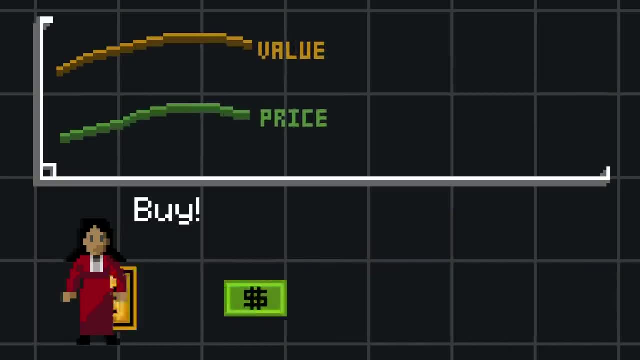 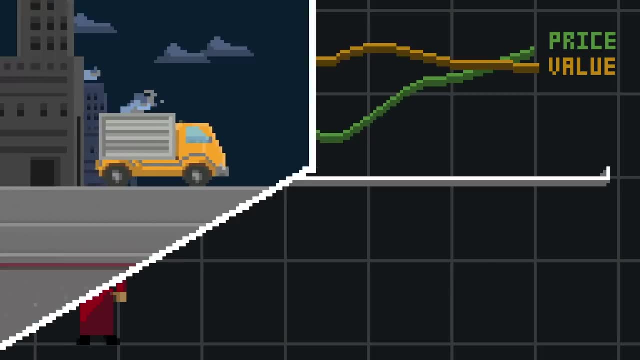 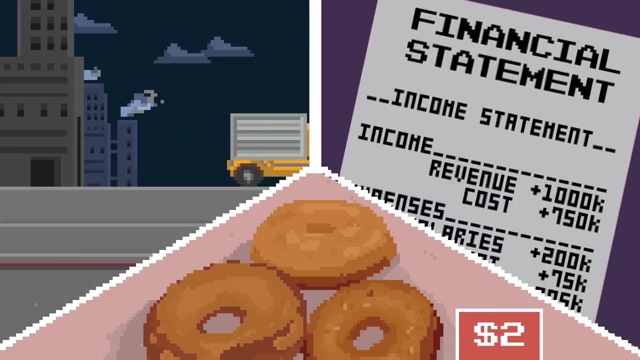 Active investors hope to exploit these inefficiencies by buying stocks they think are priced low. To identify undervalued stocks, they may investigate a company's business operations, analyze its financial statements, observe price trends or use algorithms. Passive investors, by contrast. 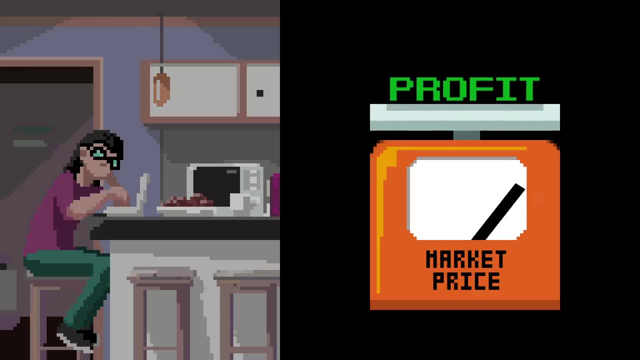 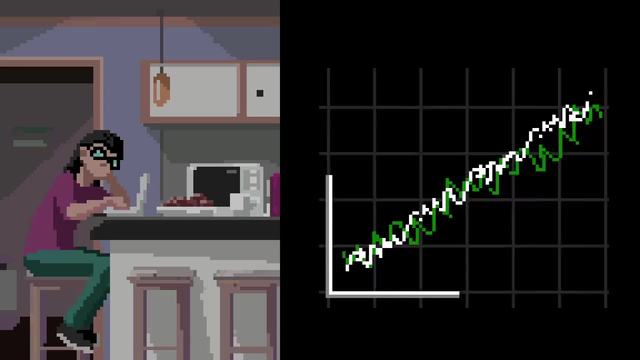 put their faith in the long-term weighing machine aspect of the market. They believe that even though markets may exhibit inefficiencies at any given point over time those inefficiencies balance out. So if they buy a selection of stocks that represents a cross-section of the market. 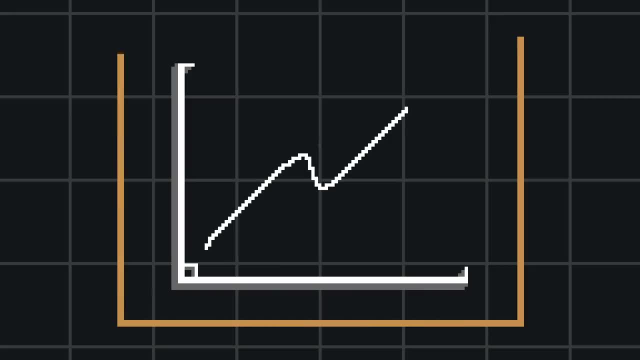 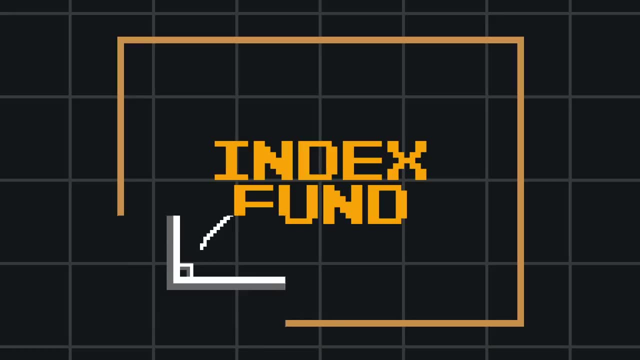 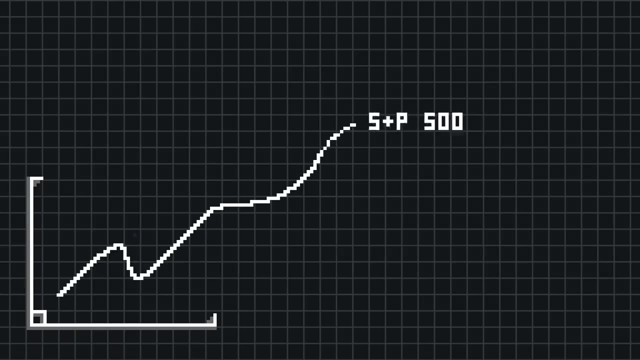 over time it will grow. This is usually accomplished through index funds collections of stocks that represent the broader market. The S&P 500 index is one of many indexes. The overall goal is the same for all index funds: to hold stocks for the long term. 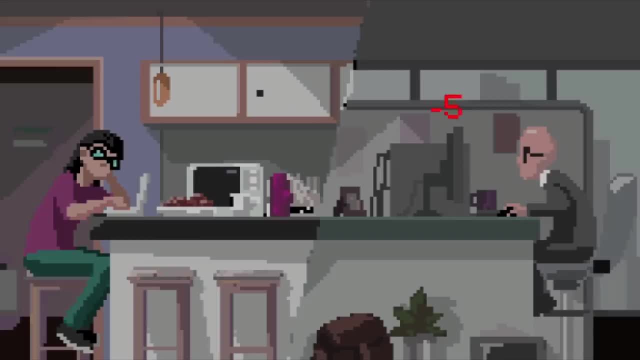 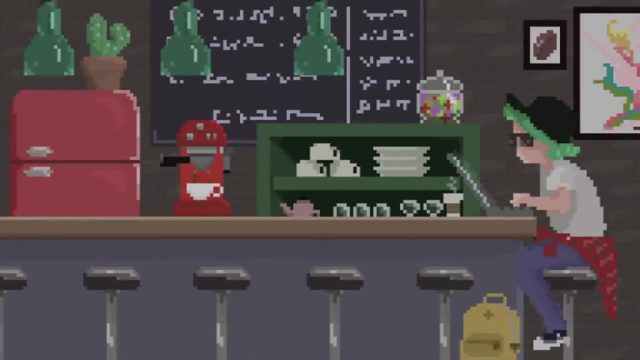 and ignore short-term market fluctuations. Ultimately, active and passive investing aren't mutually exclusive. Many investment strategies have elements of each, For example, choosing stocks actively but holding them for the long term, as passive investing advises. Investing is far from an exact science.